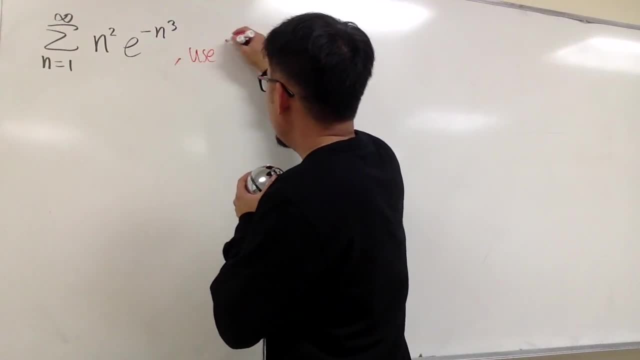 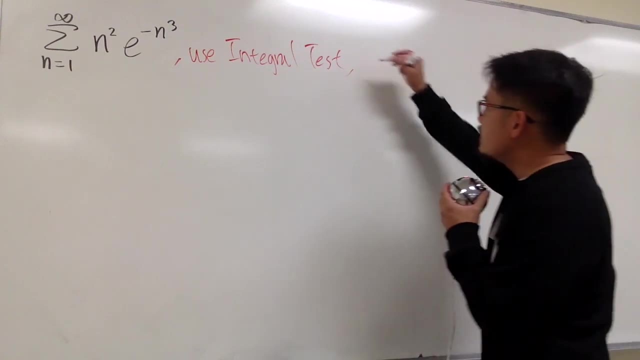 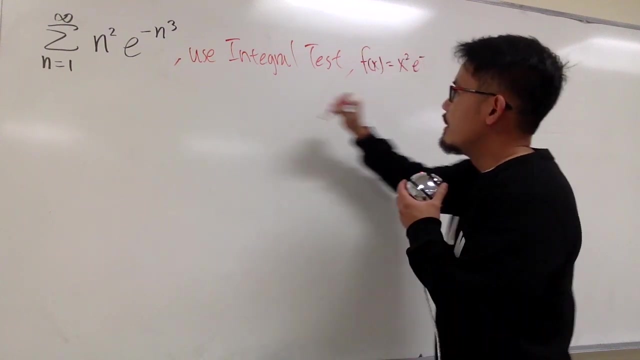 So in this case, let's attempt with the integral test And then to use the integral test, we have to first identify the function. So let me write that down: f of x, It's just x squared times e to the negative, x to the third power. 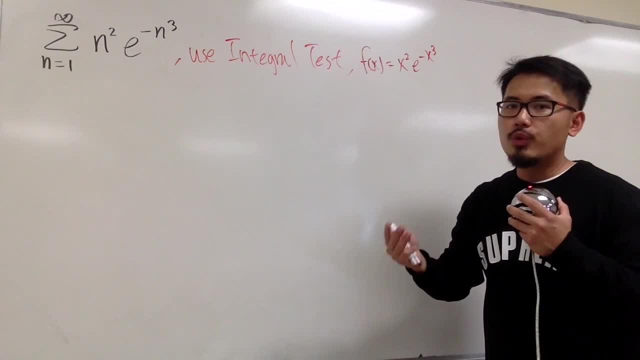 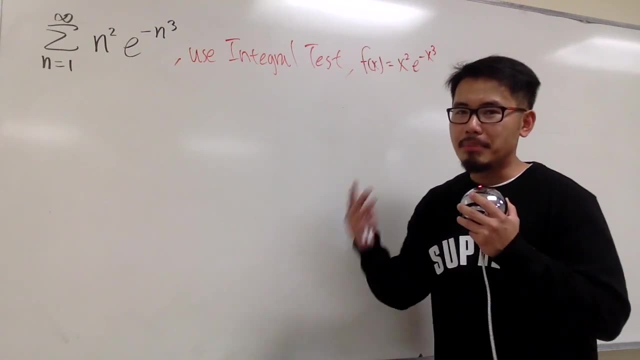 And then we have to make sure that this function has three things. We have to make sure that the function first is continuous, and then, second, it has to be decreasing, and then, third, it has to be positive. And the way you can show it is that you can just supply me with a graph. 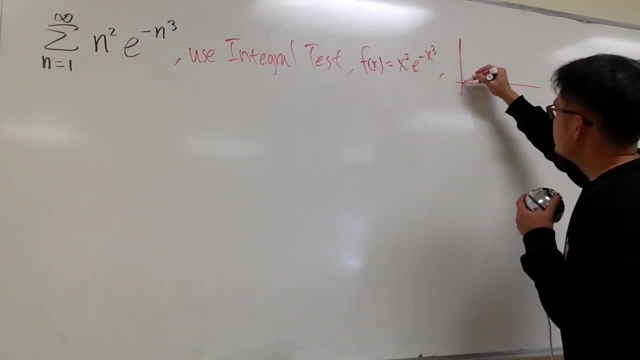 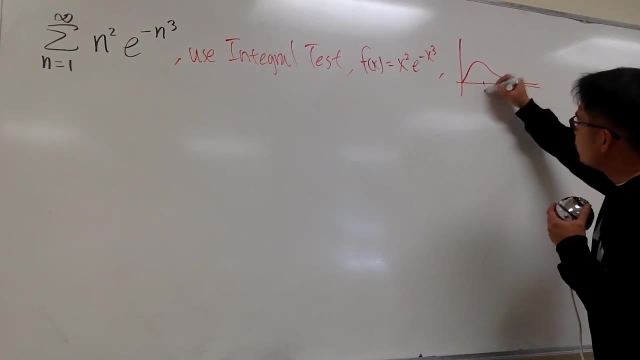 So draw a graph somewhere on the side, graph this, and we just care about the right-hand side, And then we get something that looks like this, And you see that if x is 1, which is right here- this portion of the graph is going to be, of course, continuous. 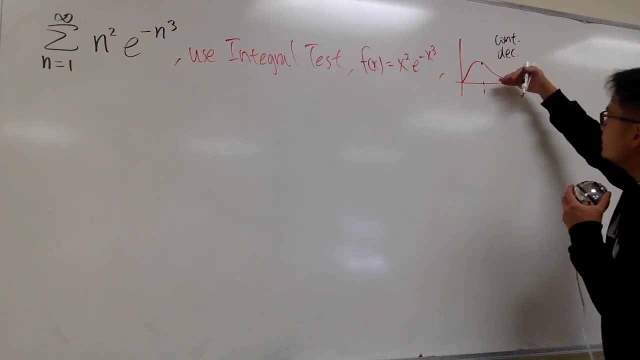 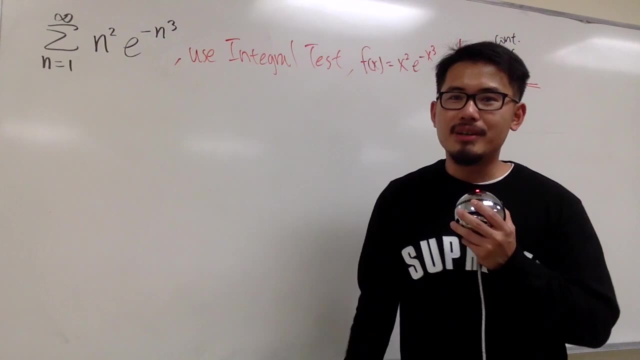 and then it's going down, so it's decreasing At the end. you know this is positive because it's above the x-axis. Anyways, we will focus on the improper integral part For the integral test. that's what we have to do. 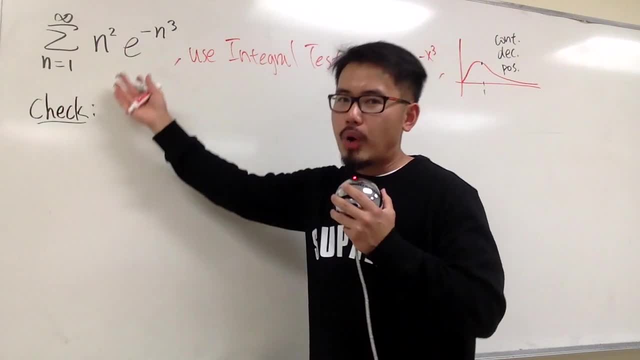 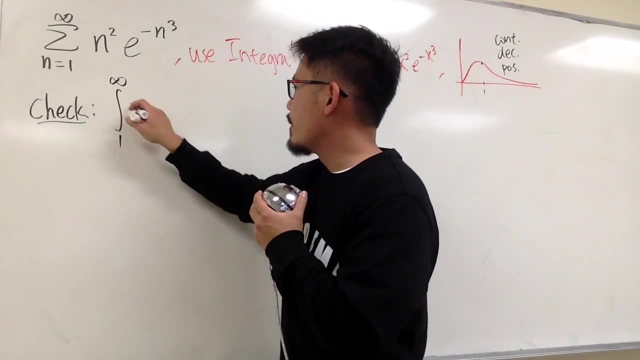 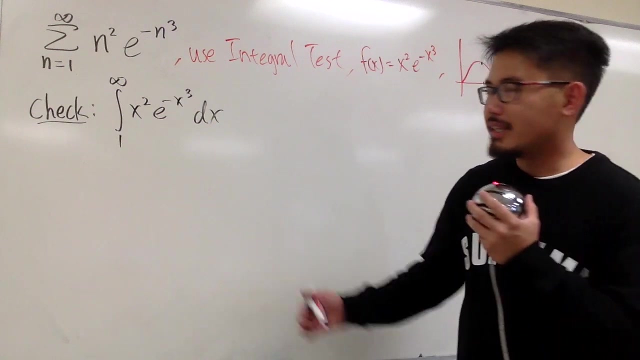 We are going to check the corresponding improper integral. So we are going to check the integral of 1 to infinity, x squared e to the negative, x to the third power, dx. The integral test says: if this improper integral converges: 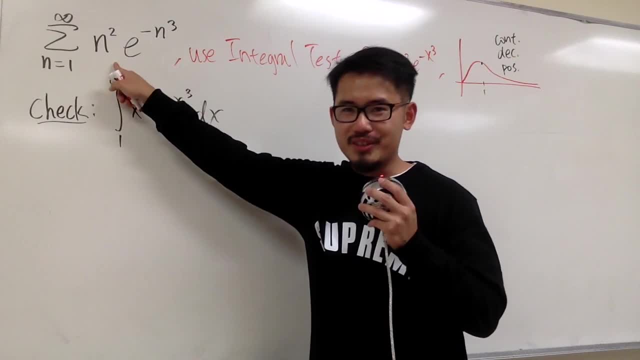 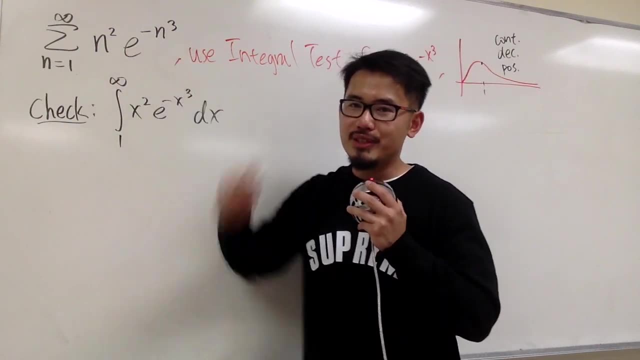 then that means this infinite series also converges, But then they may not converge to the same value. If this diverges, that also diverges. Anyways, we will integrate this. To do that, we will use U-shape. 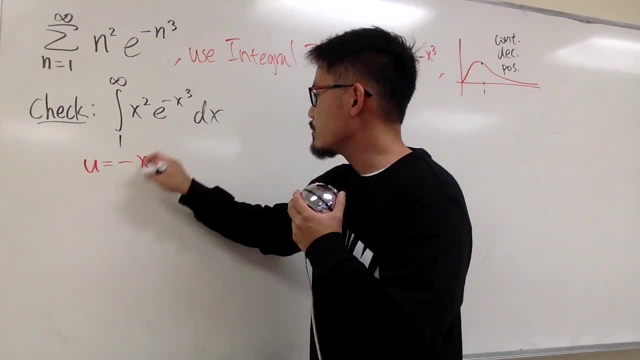 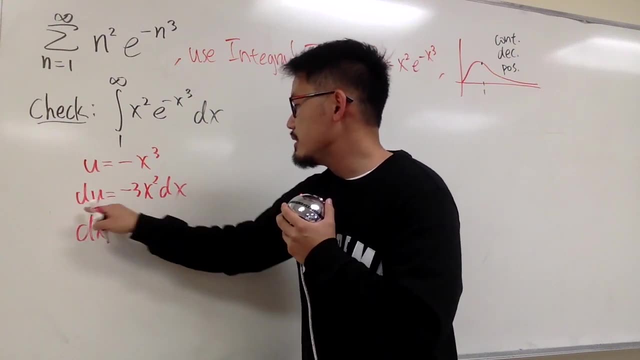 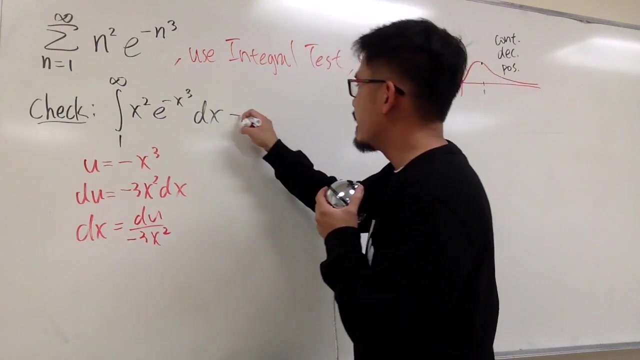 In the substitution, U is equal to the inner function, which is the negative, x to the third power, du, which is negative 3x squared dx, and isolate the dx, we get du over negative 3x squared And we take this integral into the U-world. 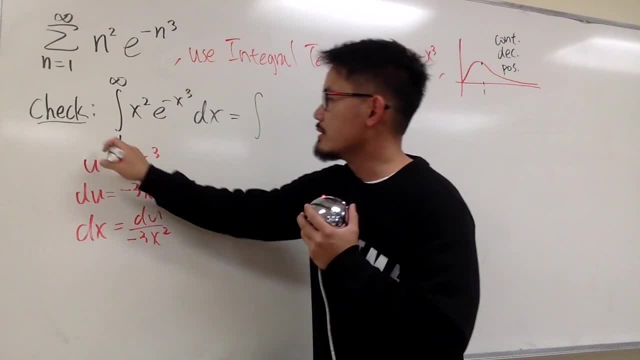 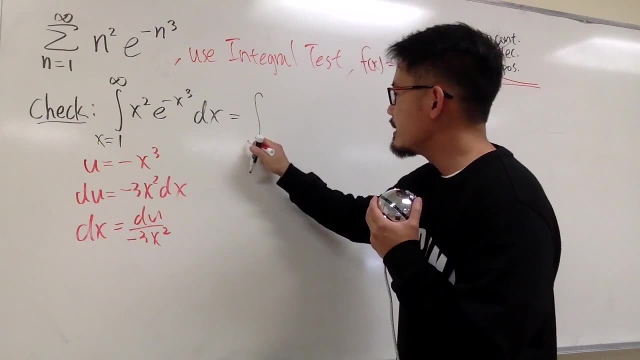 we get the integral. This is 1 in the x-world. so that means x is equal to 1.. Plugging 1 into here, we know U is equal to negative 1. to the third power, u is negative 1.. 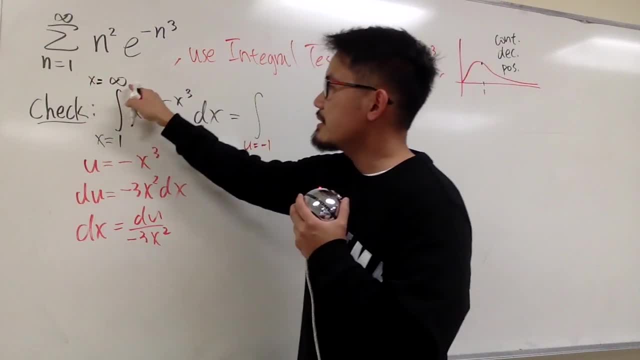 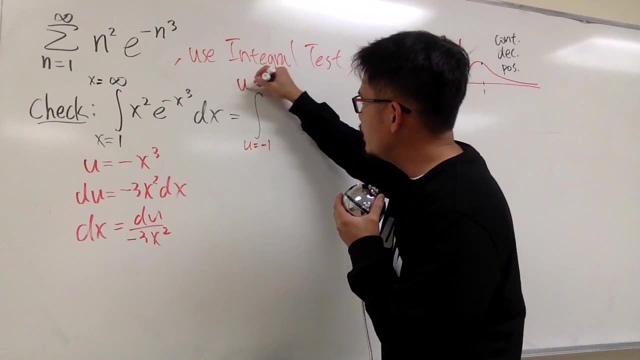 And then when we plug in this infinity, which is in terms of x, when x is infinity, plug into here we know u is equal to negative infinity, to the third power. that means u is negative infinity. x squared is just x squared. 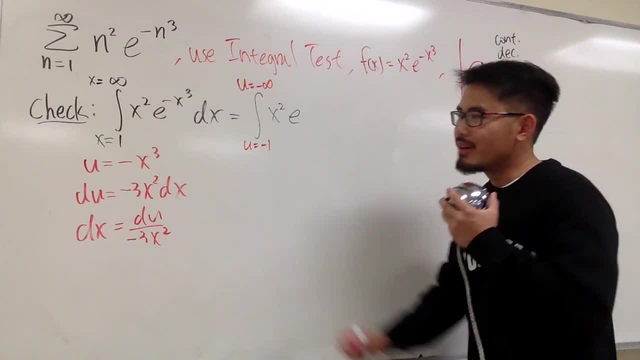 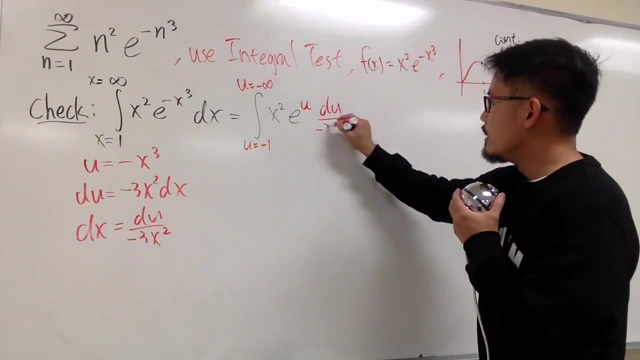 e this part. negative x to the third power is the u. So I'll just put down right here: dx is du over negative 3x squared and then, as we can see, x squared, x squared, cancel each other out. 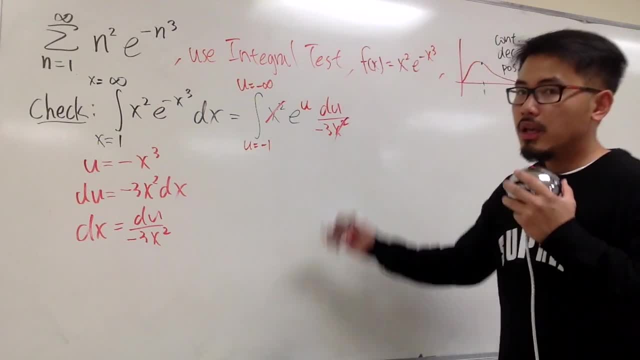 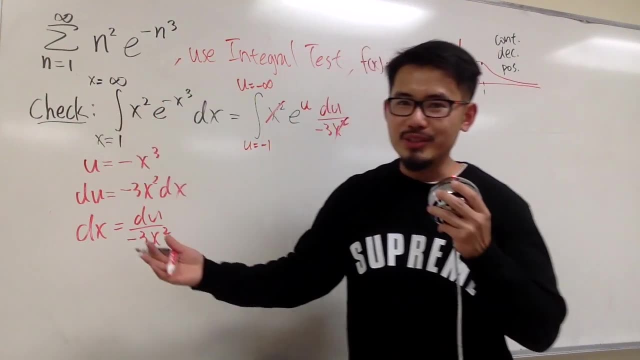 And we will just work out everything in the U-world. If this is the finite value, that means the original, improper, integral right here converges. so we focus on this. This is going to be. let me take out the 1 over negative 3 first. 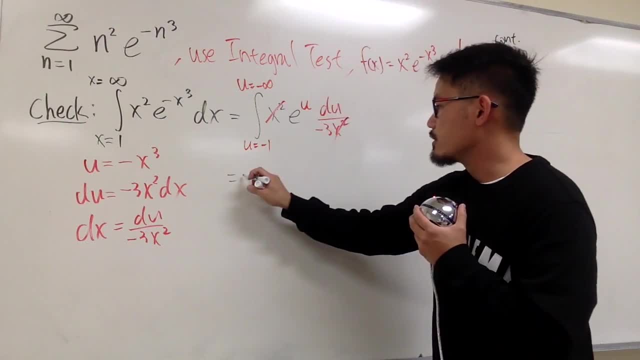 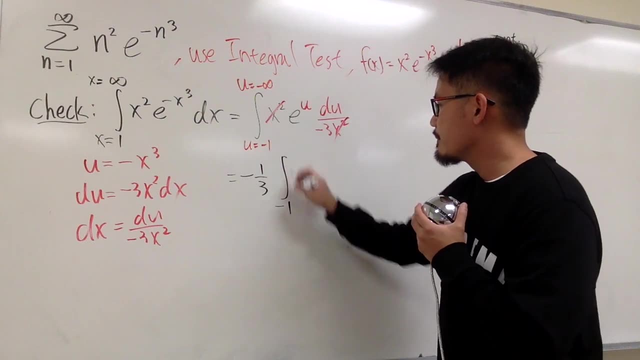 so we have negative 1 over 3 in the front and then we have the integral from negative 1 to negative infinity, e to the U-world, and then we have the integral e to the U negative infinity right here, and then e to the U du. 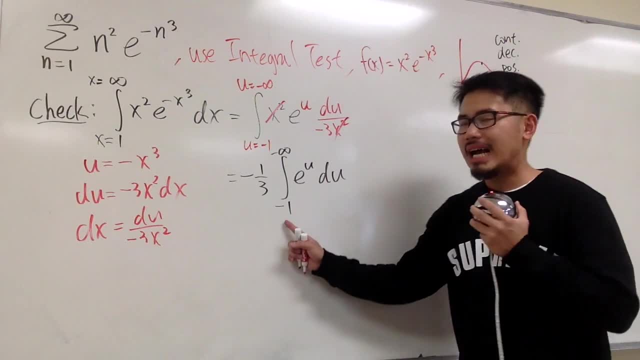 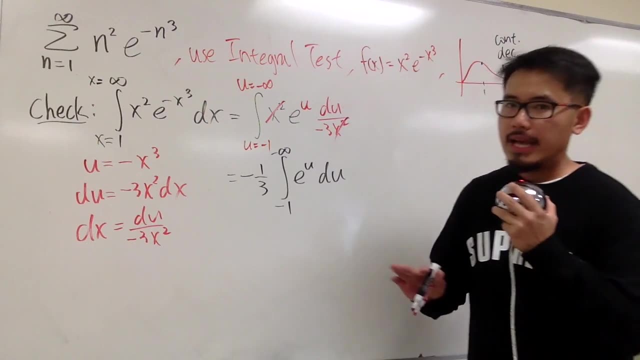 Some of you guys may notice this right now that we have a bigger number on the bottom. Negative 1 is technically bigger than negative infinity, right, But it's okay, I'm not going to do anything fancy to change this. I'm just still going to use the FTC2,. 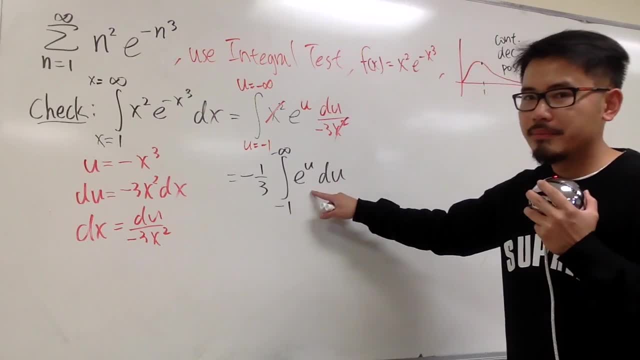 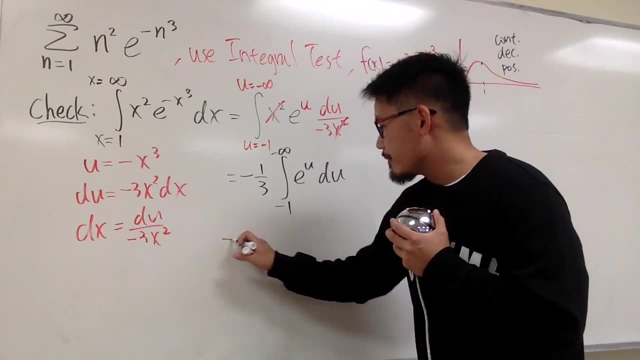 namely, we are going to first find the antiderivative of this and then plug in the upper number right here, subtract, after we plug in the lower number, just in that order. that's all. Anyways, let me remain the negative 1 over 3 in the front. 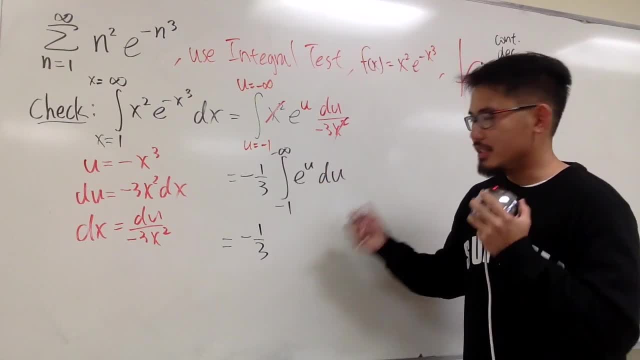 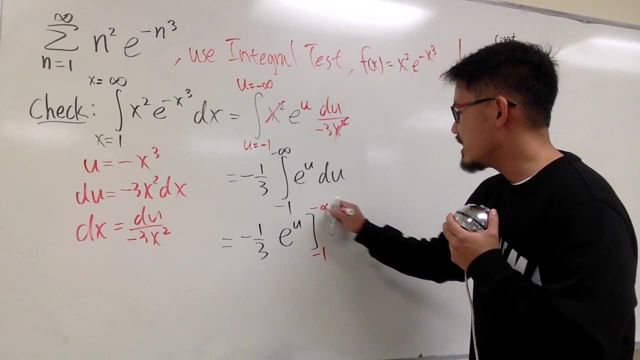 and then the antiderivative of e to the U in the U-world is just e to the U. so we did the integration and then we have to plug in values. now it goes from negative 1 to negative infinity. and FTC2 says: 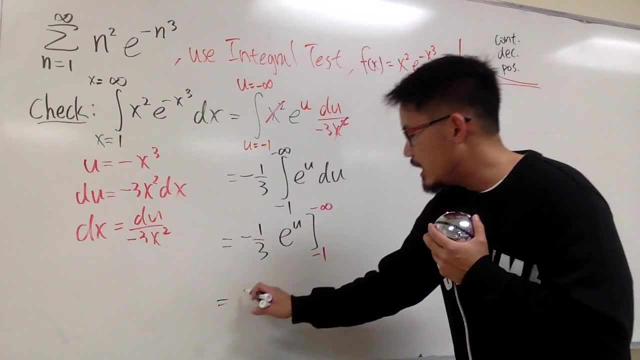 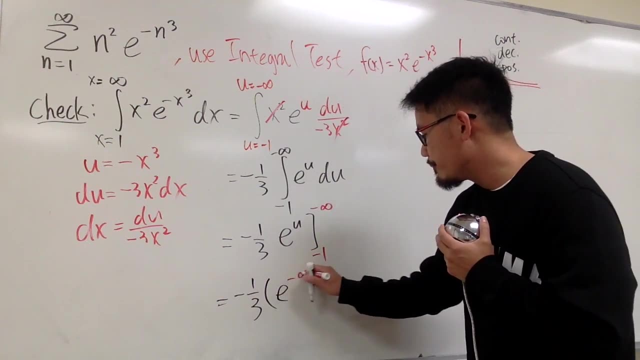 I'm just going to plug in negative infinity into U first, and then we keep the negative 1 third all the way in the front first, and we will have e to the negative infinity, and then we subtract, we plug in negative 1 into that.